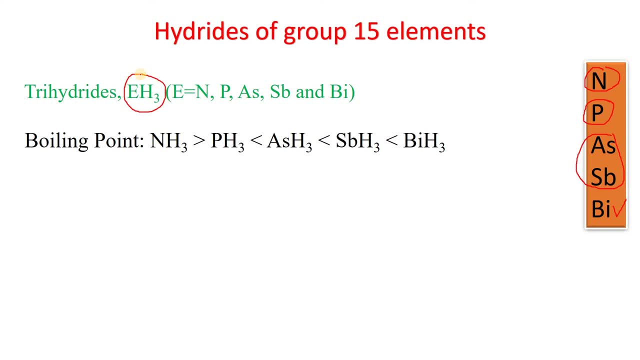 If we discuss about the boiling point, the trend in the boiling point: the hydride of nitrogen, trihydride of nitrogen, which is popular name ammonia, has a boiling point higher than pH 3, phosphine, And then the phosphine has lesser boiling point than arsine. and then stebin, and then bismuthine. 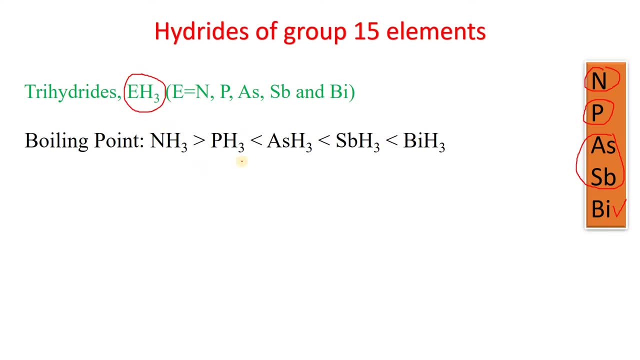 So there is no regular trend in the boiling point of the hydride of the trihydride of the group 15 elements. The ammonia has larger boiling point than phosphine is due to the strong hydrogen bonding which exists in the ammonia and the NH3 molecule are associated strongly. 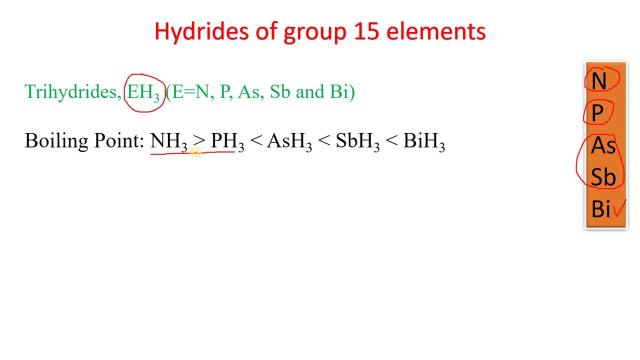 So, due to strong hydrogen bonding, the ammonia has higher boiling point than the pH 3.. But as we go from fast force to bismuth, the boiling point is again increasing. This attribute duty increase in the size of the central element, which increases the non-covalent interaction. 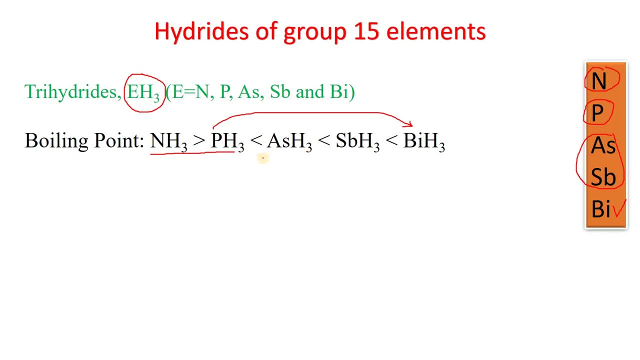 So that's why the boiling point again increases from phosphine to BIS3.. The thermal stability: if we talk about the thermal stability of the molecule, the thermal stability decreases as we go from Ammonia to BiH3. The BiH3 molecule is not very stable. 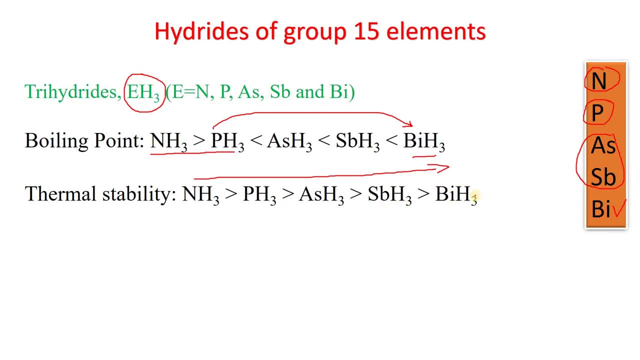 The stability is upto SbH3. The BiH3 molecule is highly unstable molecule. The thermal stability decreases from Ammonia to BiH3, So Ammonia is maximum stable among these hydrides. What is the reason behind this? The covalent bond enthalpy, the bond enthalpy, the bond strength of Ex bond is like this: 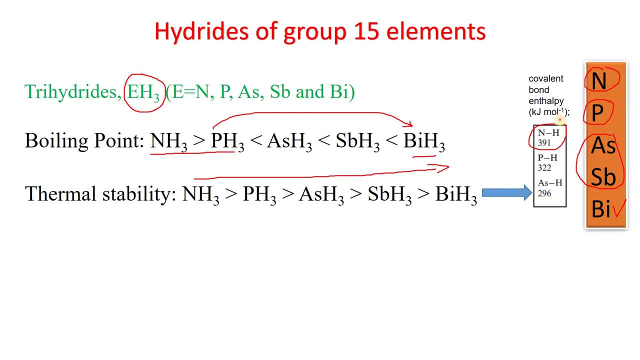 The Ns bond is the bond energy of bond enthalpy is 391 kJ per mole. Down the group it decreases 322 and it is 296. That's why the thermal stability decreases going from Ns3 to BiH3, The basic reactor. basic reactor means the tendency to donate the lone pair of electrons present on the central atom E. 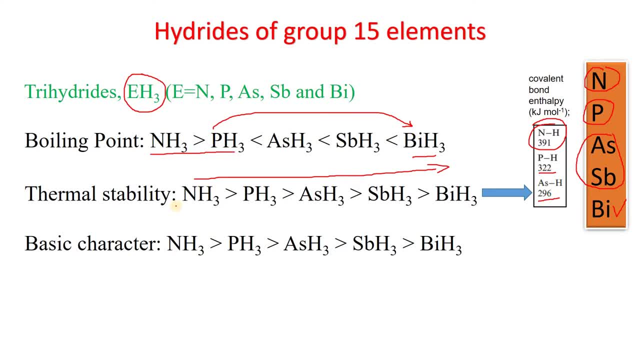 towards a Lewis acid. So the basics or the basic reactor is: decreases Ns3 as a lone pair, nitrogen then Phosphose, also lone pair, then Arsenic and Timonic. So the covalency or the tendency to donate these lone pair of electrons to some Lewis acid. 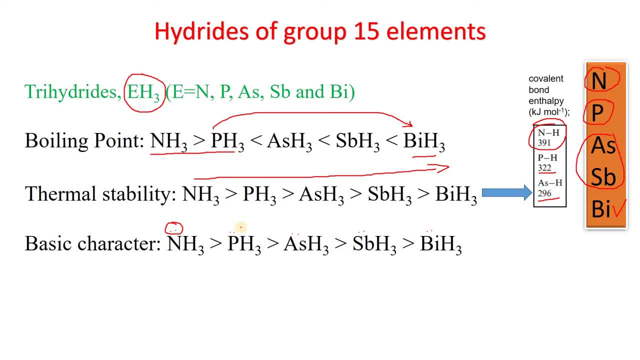 So the covalency or the tendency to donate these lone pair of electrons to some Lewis acid is decreases as we go from Ns3 to BiH3. This is the trend in the basic reactor. So the lone pair are mostly available on the nitrogen in case of Ammonia. 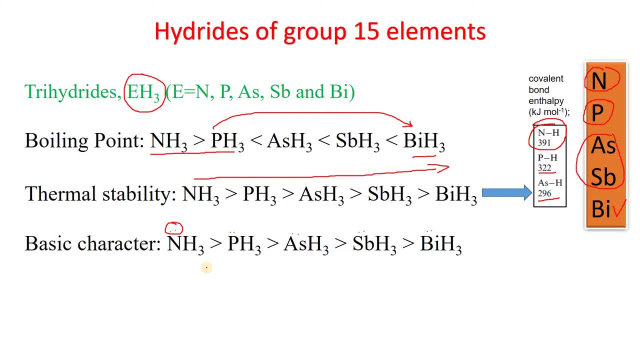 and it is least available on Wismuth. in the case of BiH3, The reducing reactor is following the reverse order as the basic reactor. As we know, the Ex bond strength is decreases from Ammonia to BiH3. That's why the BiH3 is the strongest reducing agent. 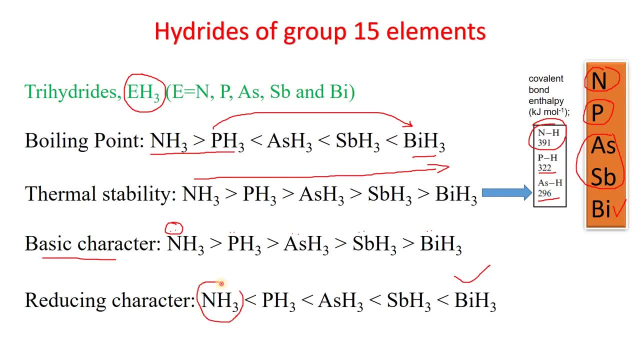 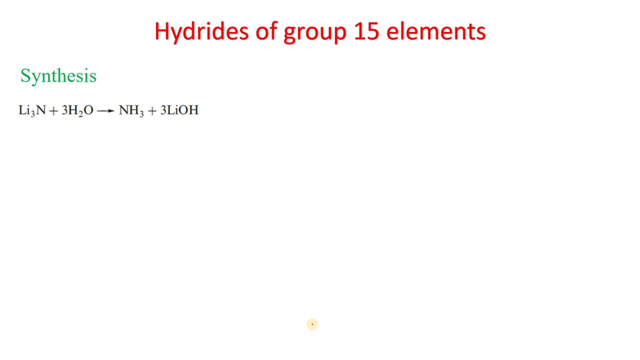 and the Ammonia is the least strong reducing agent. Then synthesis part. How can we synthesize the hydride or 15 group element? For the synthesis of Ammonia? we can use Lithium Nitride and hydrolysis with the water molecule produces the Ammonia. 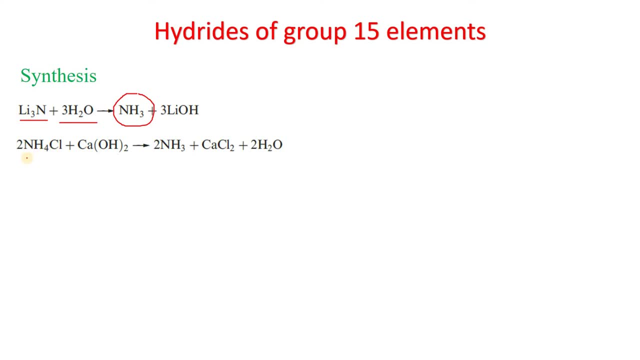 Another method is by using the Ammonium chloride and calcium hydroxide. The Ammonia is produced. We can reduce the Zinc and Nitrate salt with Zinc in the basic medium and we will get the Ammonia. Another method or a general method for the preparation of hydride: 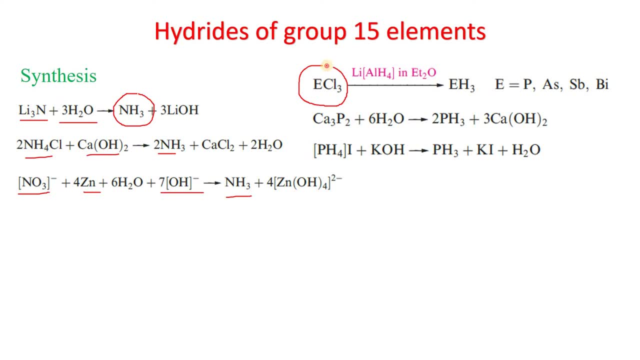 We can take the ECl3 type salt like PCl3, ACl3 and reduce with the Lithium Aluminium Hydride in diethyl ether. We will get the EH3. where is Phosphose, Arsenic, Antimony and Wismuth? 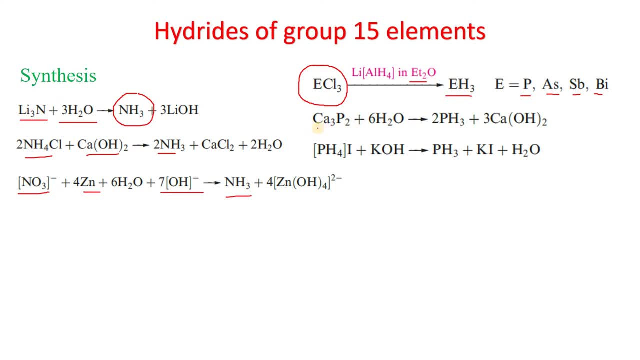 We can similarly use Calcium Phosphate, Ca3P2 Hydrolyze with water and we will get the Phosphine And the another. we can use the iodide salt with Potassium Hydroxide and we also get the Phosphine. The commercial synthesis of Phosphine uses the disproportionation. 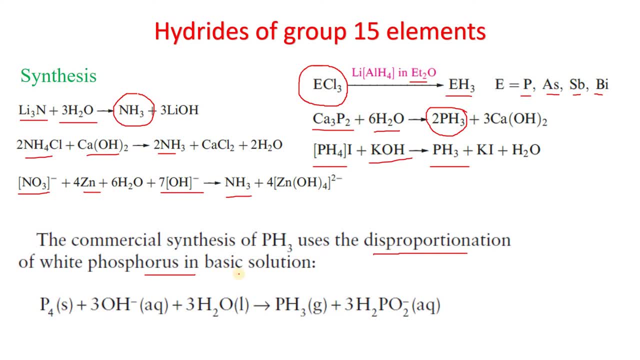 of white Phosphores in the basic solution. Disproportionation means the same molecule is oxidized and reduced. So Phosphores, Elemental Phosphores, when treated with water in the basic medium we get the Phosphine gas and the F2PO2- in the aqua source. 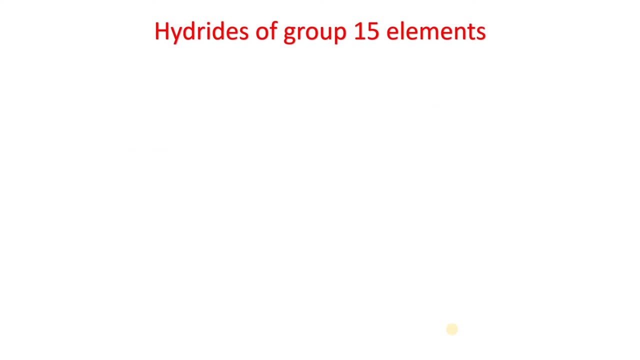 The industrial manufacture of Ammonia, which is very important, involves the Haber process. Haber process is a well known process which is used for the production of Ammonia, and Ammonia is very useful compound which is further used for the manufacturing of manufacturing of fertilizers. 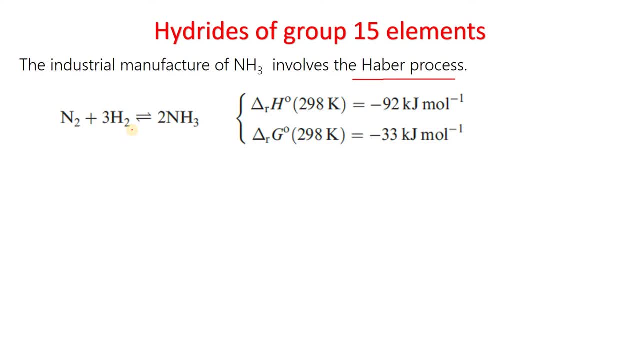 The 1 mole of Nitrogen. when treated with the 3 mole of Nitrogen we get the 2 mole of Ammonia. This is a reversible reaction and the delta H is negative. the reaction is exothermic and delta G is also negative means the reaction is feasible. 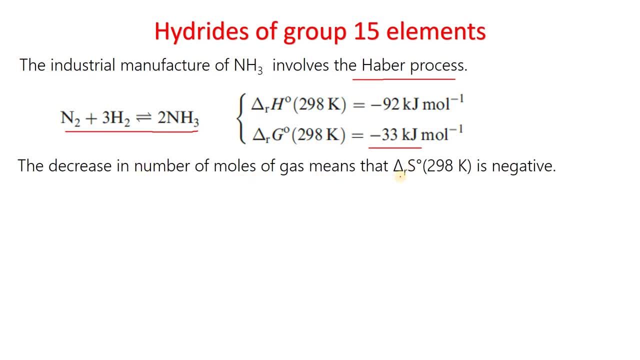 But the decrease in the number of moles of gas means that entropy is negative, which is a problem. So the number of moles in the reactant are 3 plus 1 is 4 and the number of moles in the product are 2. 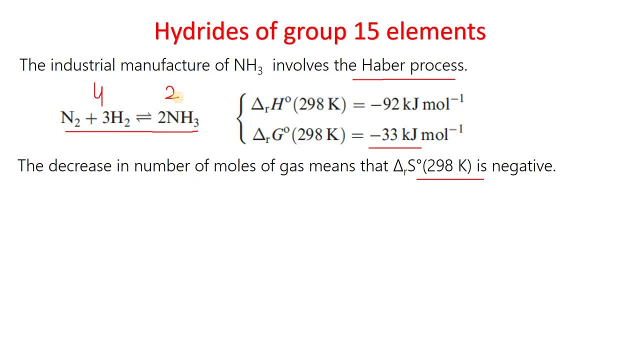 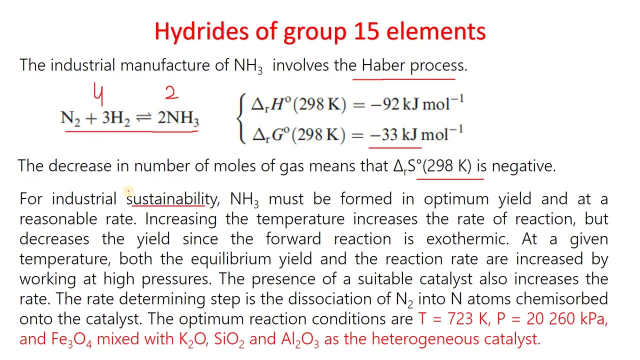 So the entropy change is 2 minus 4 minus 2, which is negative. So for the industrial sustainability, for the industrial purpose, Ammonia must be formed in optimum yield and at a reasonable rate. So for the industrial purpose, we require both things. First, the rate should be fast. 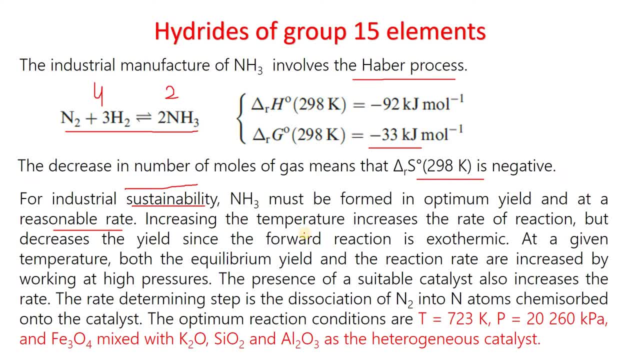 and the yield should be high. But, as we know, this is an exothermic reaction. If you increase the temperature, then the rate of reaction decreases. Increasing the temperature increases the rate of reaction. When you increase the temperature, it increases the rate of reaction but decreases the yield. 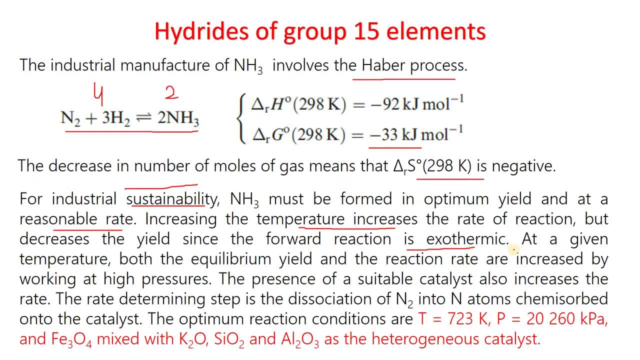 since the follow reaction is exothermic, So for at a given temperature both the equilibrium yield and reaction rate are increased by working at high pressure. So the optimum conditions are The temperature, 723 Kelvin, Pressure, 20260 kilopascal, And we use the catalyst Iron oxide, Fe3O4. 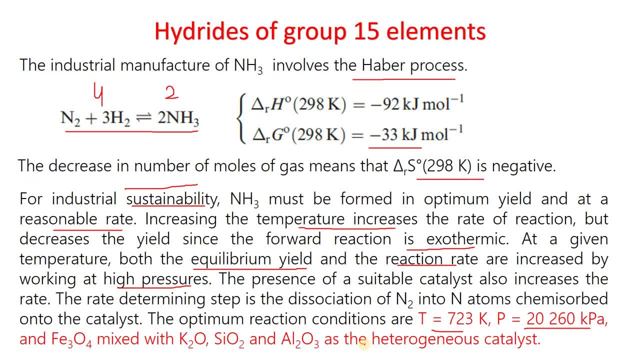 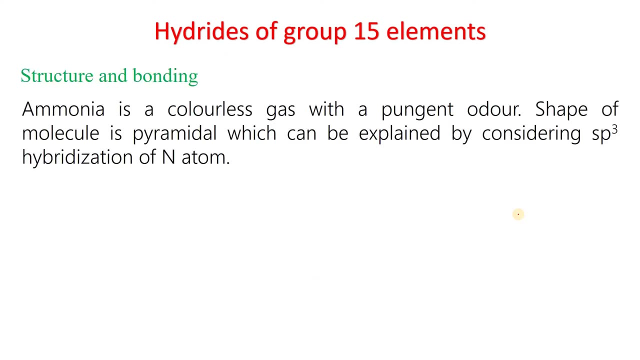 mixed with potassium oxide and aluminium oxide as the heterogeneous catalyst. So industrially, the ammonia is produced by the nitrogen and hydrogen in the presence of the catalyst at this temperature and this much pressure. Then come to the structure and the bonding part. Ammonia is a colorless case. 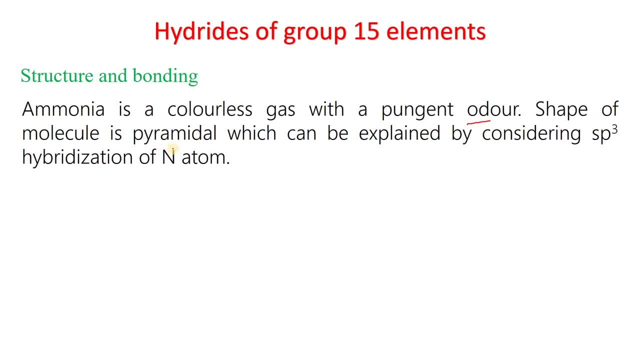 with a pungent odor. The shape of the molecule is pyramidal, which can be explained by considering the sp3 hybridization of the nitrogen. As we know, the nitrogen has the electronic configuration. The valence cell electronic configuration is 2s2 and 2px1. 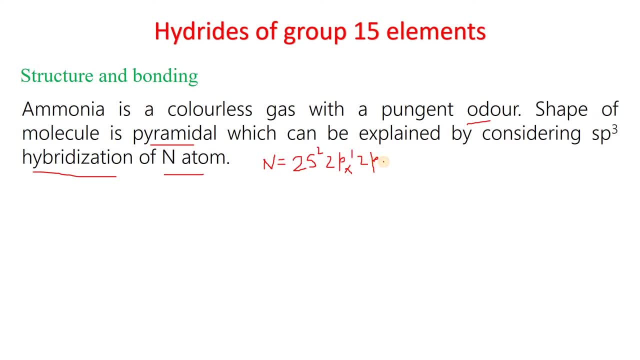 2py1 and 2pz1. So in the valence cell there are 4 electrons, sorry, 5 electrons. on the nitrogen atom, If we consider the sp3 hybridization, If we consider there is 1 electron and there are 2 electrons, So sp3. 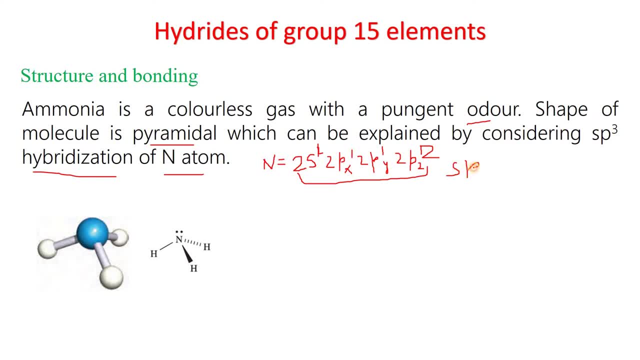 So there are 4 sp3. So these 2 electrons will remain in either of the orbital, either in 2pz or in 2py, or 2px or 2s. So upon hybridization we are getting 4 sp3 hybrid orbital, out of which 3 are singly occupied. 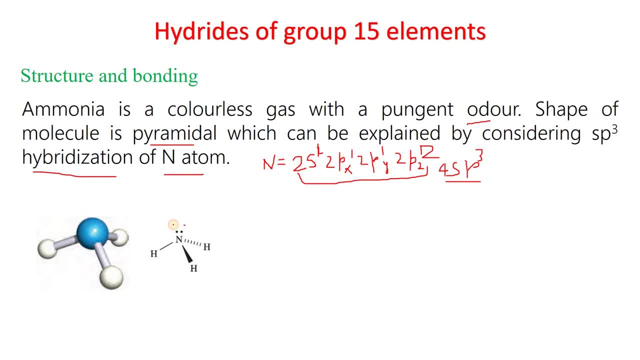 and one is doubly occupied and this lone pair is present in one of the sp3 orbital and these 3 single electrons will form the bond with the hydrogen atom, the 1s orbital of the hydrogen atom, and this is a pyramidal shape like this: 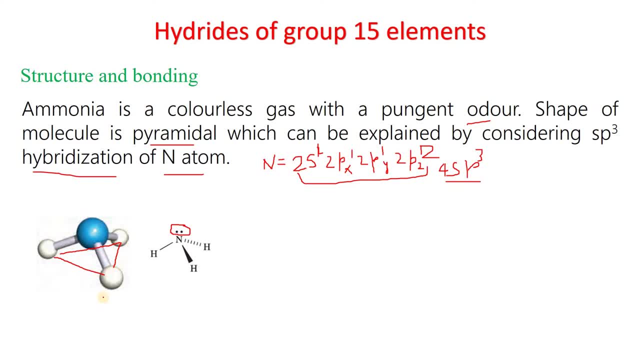 this is a form of a triangle and at the center of triangle, above the plane of the triangle, there is nitrogen, and so the shape of the ammonia is pyramidal- pyramidal. and ammonia is a water soluble, weak base. the acidity, or basicity, can be measured by the pKa and pKb values. 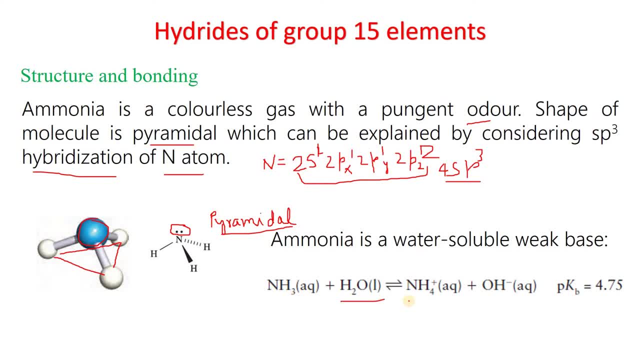 when ammonia is dissolved in water- liquid water- we will get the ammonium ion and the hydroxide ion, and this hydroxide ion is the cause of the basicity of the ammonia and the pKb value is 4.75, which indicates the ammonia is a weak base in the water. 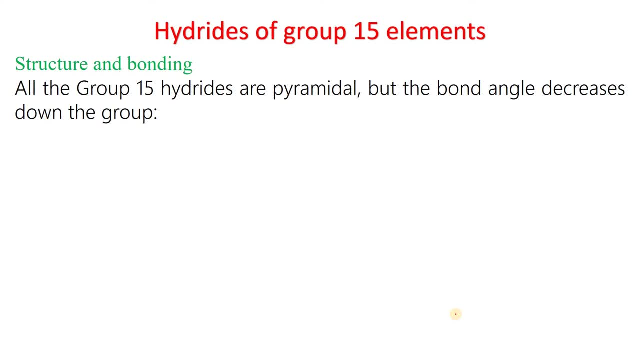 and all the group 15 hydrides are pyramidal, like ammonia, but the bond angle decreases down the group. so the maximum bond angle is observed in ammonia ns3 and the least bond angle is observed in the biH3. why this trend? so in ammonia the angle is around 108 degree. 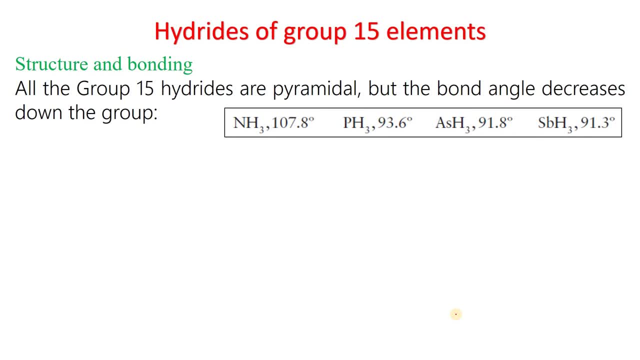 but as we are going down the sbH3, the angle is 91.3 degree. we are not considering the biH3 here because the biH3 molecule is highly unstable molecule. so not much data is available for biH3. so we are talking about the four molecule only. 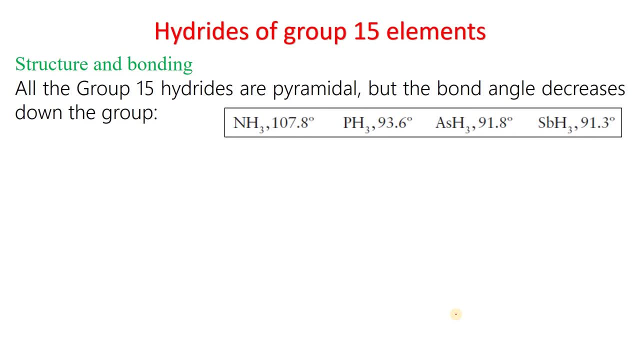 ns3, ph3, aish3 and sbH3. so the bond angle is: decreases down the group. so if we draw the structure like this, E molecular pyramidal H, where E is either nitrogen or phosphorus or arsenic or antifree, this is a lot. 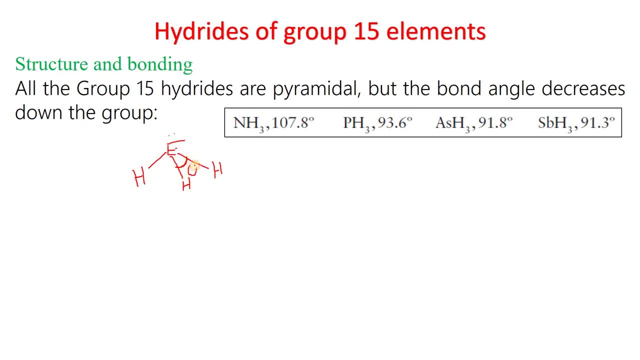 so this angle is suppose theta, and this angle is decreases from approximately 108 degree to 91.3 degree. what is the reason behind this? the bond pair in the E-H bond are responsible for this trend. as in case of ammonia, the size of nitrogen is small. 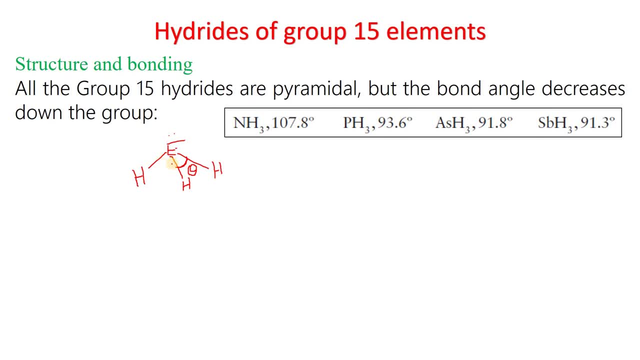 so these bond pair are very close to each other and that's why they are repelling to each other. so we are getting the maximum value of bond angle in case of ammonia. but as we go to the S sbH3, the size of the central atom is: 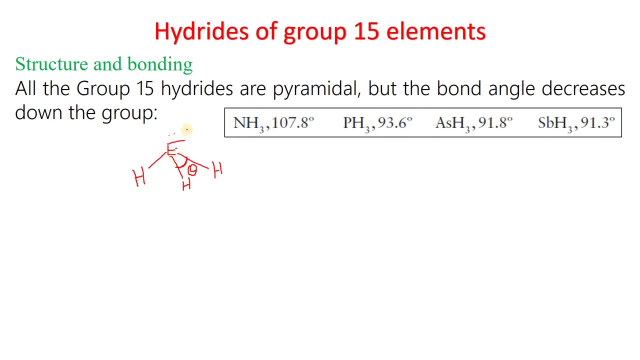 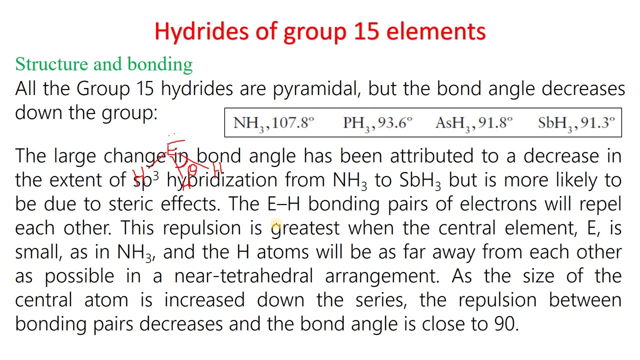 increases and the repulsion between the E-S bond pair is decreases and we are getting the smaller bond angle in case of SbH3. so the large change in the bond angle has been attributed to a decrease in the extent of sp3 hybridization from ammonia to SbH3. 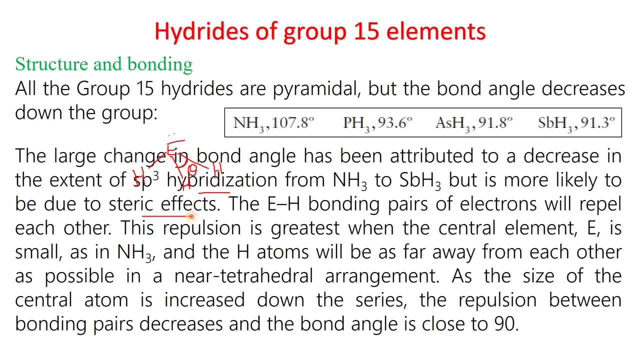 but is more likely to be due to the steric effects. the E-S bonding pair of electron will repel each other. this repulsion is greatest when the central atom E is small- that is, ammonia- and as we and the hydrogen atom will be as far away from each other. 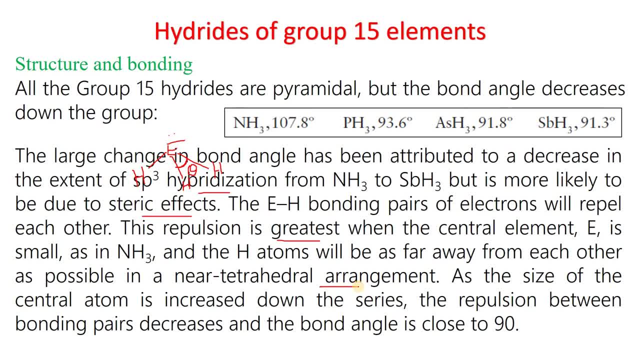 as possible in near tetrahedral arrangement. as the size of the central atom is increased down the series, the repulsion between bonding pair decreases and the bond angle is close to 90 degree. so the repulsion is the main cause for this trend in the bond angle. 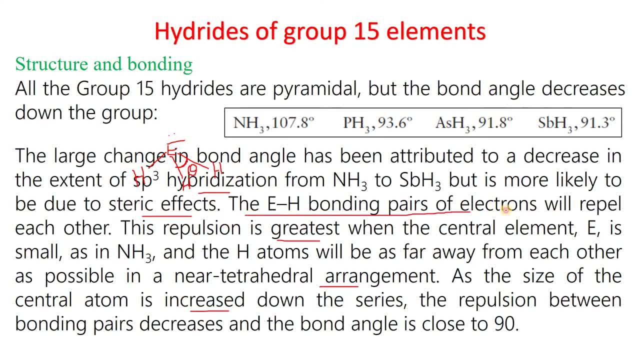 so when the E-S bonding pair of electron will repel each other. so when the size is small, the size of E is small, there is maximum repulsion between the bonding pair and we are getting the maximum angle. but as we are going down the group, the size of the central atom E. 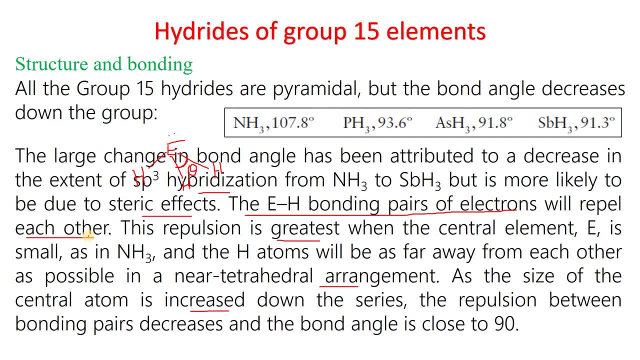 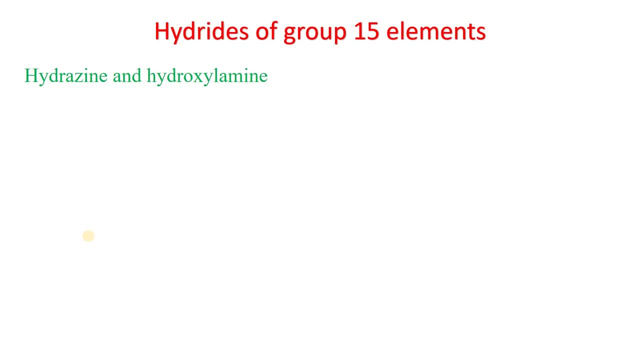 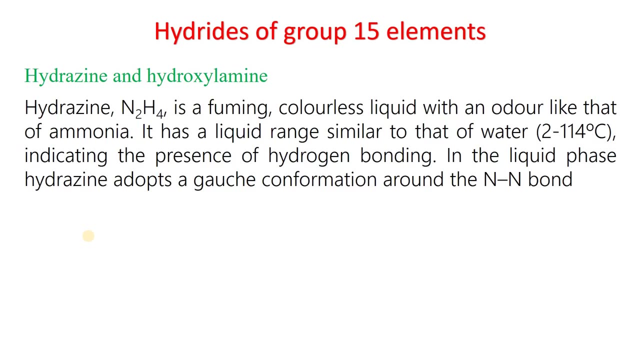 increases, and this repulsion is also increases, and that's why the repulsion is decreasing and the bond angle is decreasing. then come to the next hydrides of the elements: the hydrazine and the hydroxyl amine. the hydrazine: 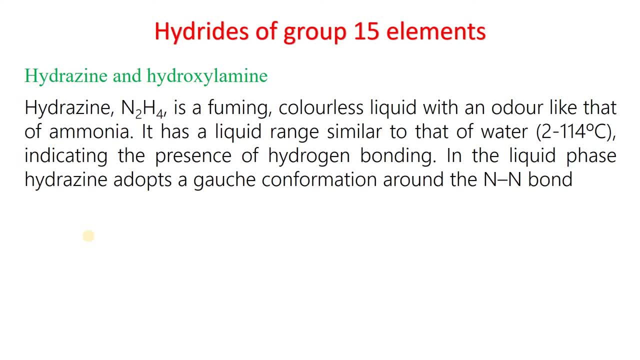 with formula N2H4 or NH2NH2 is a fuming colorless liquid with an odor like that of ammonia. it has a liquid range similar to that of water, from 2 to 1.4 degree centigrade, indicating the presence of hydrogen bond. 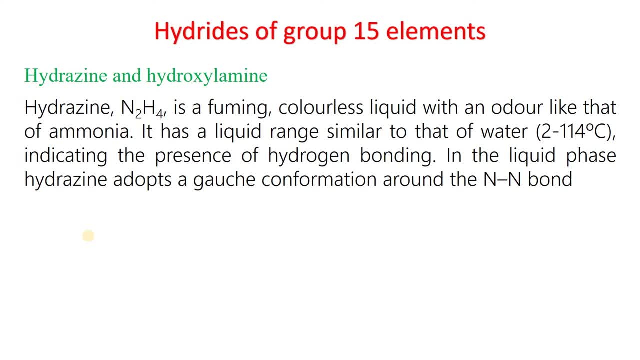 in the liquid phase. hydrogen adopts a gross conformation around the nitrogen nitrogen bond like this: this is blue color is nitrogen and the white color are the hydrogen. so the angle is 95 degree and this angle HNH is 108 degree and the nitrogen and nitrogen. 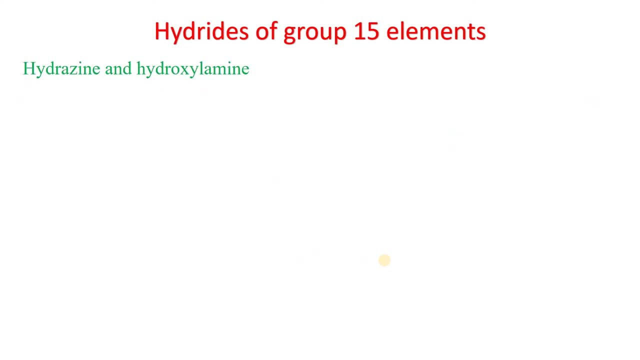 bond length is 145 picometer. how? how we will synthesize the hydrogen. this process is known as pressing process. ammonia- aqueous ammonia is created with sodium hypochlorite and we get NH2Cl and sodium hydroxide and in the next reaction, ammonia reactivate. 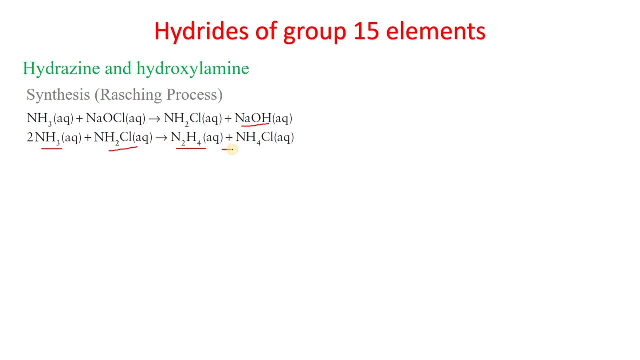 NH2Cl and we will get the N2H4 in the aqueous solution and hydrogen bond and hydrogen is weaker base even than the ammonia. when dissolved in water we get, we will get the hydroxide ion. PKB1 is 7.93. 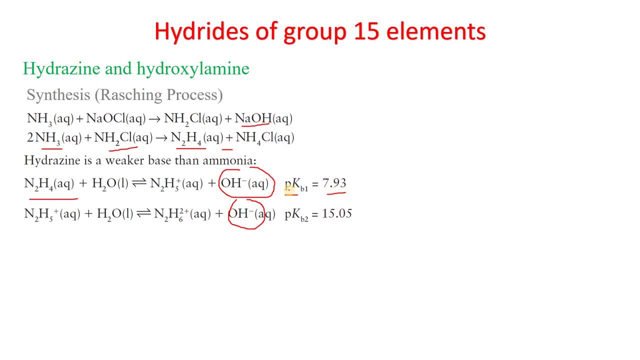 the ammonia has PKB of 4.75. it is even weaker than the ammonia, and PKB2 value is even less. even more so the overall, the hydrogen is a weaker base than the ammonia. the major use of hydrogen and its methyl derivative, like CH3NHNH2. 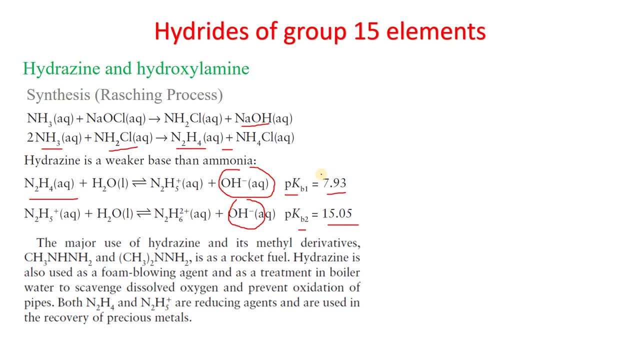 and CH3NNH2 is as a rocket fuel. hydrogen is also used as a storm blowing agent and as a treatment in boiler water to cleanse dissolved oxygen and purvate oxygen of the pipes. both hydrogen and N2H5 plus are reducing agent and are used 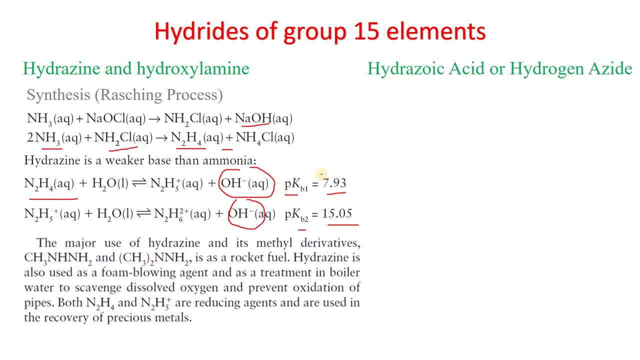 in the recovery of the precious matter. and next, hydride is hydrozoic acid, or known as hydrogen azide. SN3 is acidic in the nature. it behaves both as an oxidizing as well as reducing agent. the azide ion has 16 electrons and is 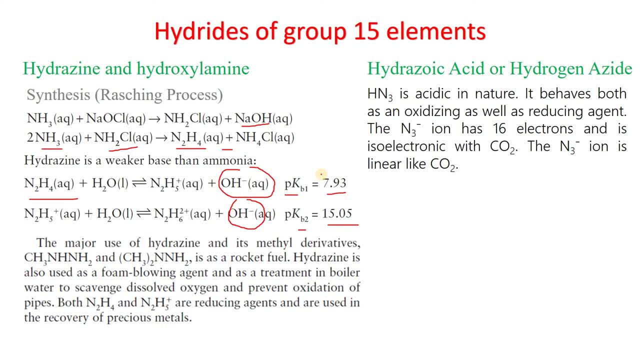 isoelectronic with isoelectronic with carbon dioxide. so structure of the hydride is very similar to the CO2. it is a linear molecule. this is hydrozoic acid. the NN distances are different. it is 1.13 and 1.24. 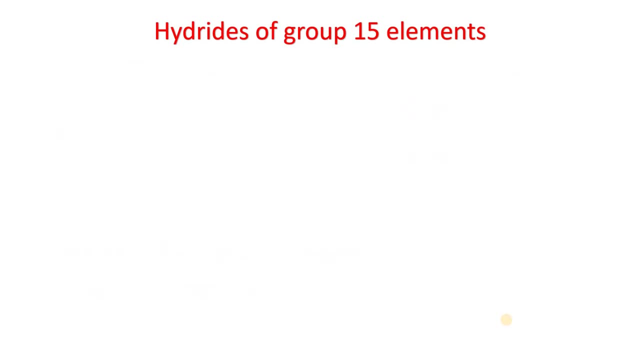 and this is the resonance, one of the resonance structure of the hydrozoic acid. so this is the structure. the blue ball are nitrogen and the white ball is the hydrogen, the. here the bone length and the bone angle are shown. here the angle is 114 degree. 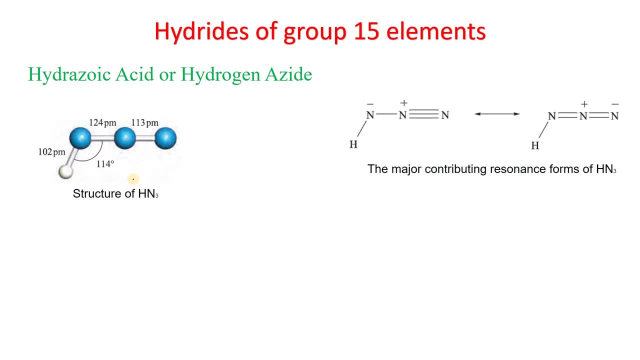 and the NH bone distance is 102 picometer and this is the structure of the hydrozoic acid. so this is one and this is two. if we move these electron pair here and these electron pair here and we will get the second resonance structure and this is. 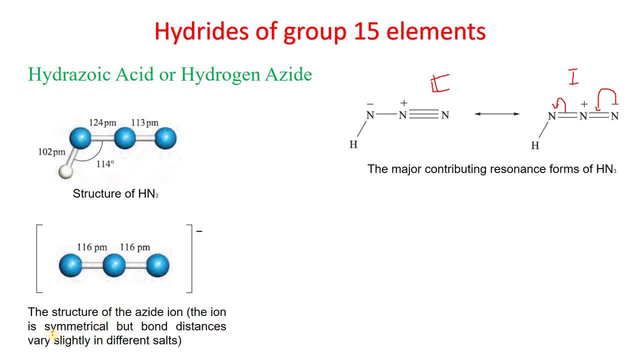 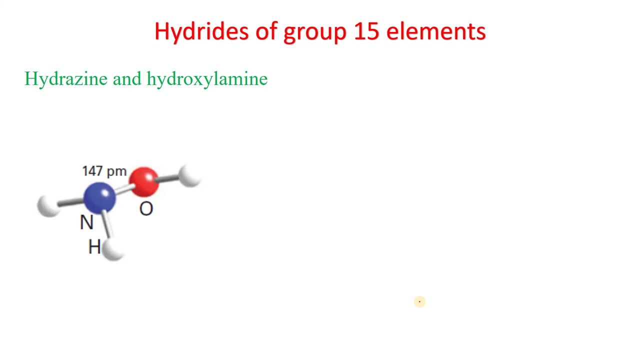 the structure of the azide ion. the structure of the azide ion: the ion is symmetrical, but bone distances vary slightly. and this is the structure of the hydrogen and hydroxyl amine. the next molecule is hydroxyl amine. we have already discussed 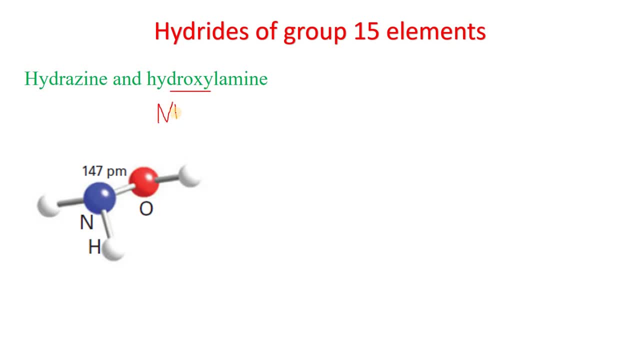 about the hydrogen. the next molecule is hydroxyl amine with the formula NH. the three dimensional structure of the hydroxyl amine molecule: the blue color is nitrogen, the red is oxygen and the other white colored balls are representing the hydrogen atoms, hydroxyl. 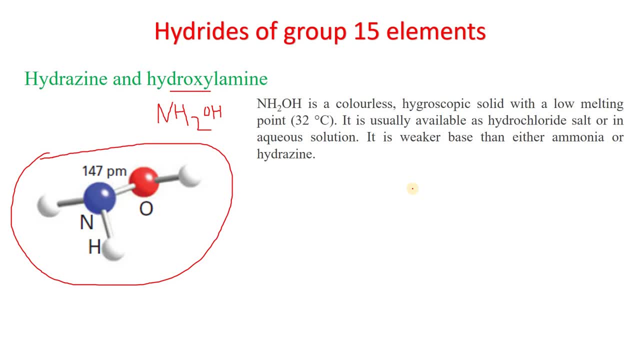 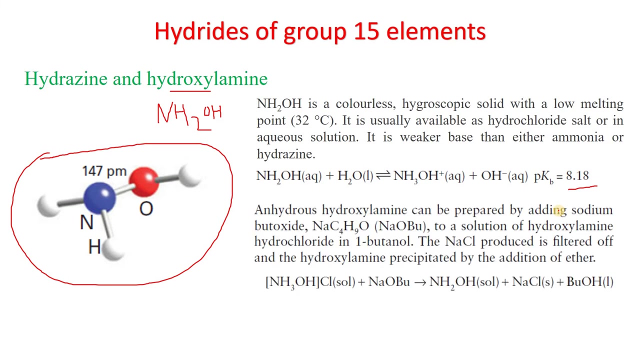 amine is a colorless, hygroscopic solid with a low melting point, like ammonia and the hydrogen, as we have discussed earlier. when it is dissolved in water, the pKb value is 8.18, which indicates it is even weaker base than ammonia and the 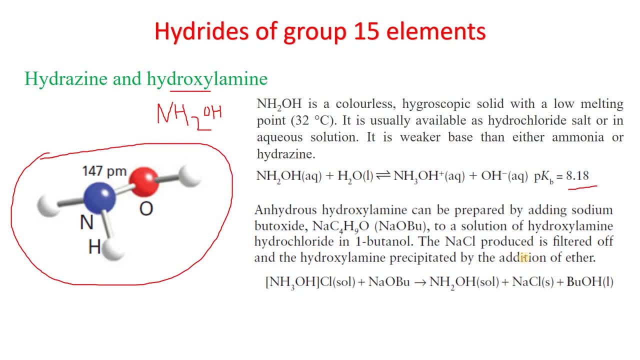 hydrogen. the anhydrous hydroxyl amine can also be prepared by adding the sodium butoxide. this is sodium to OH in the solution and NCl is separated out, filtered off and the hydroxyl amine precipitated by addition of the ether. 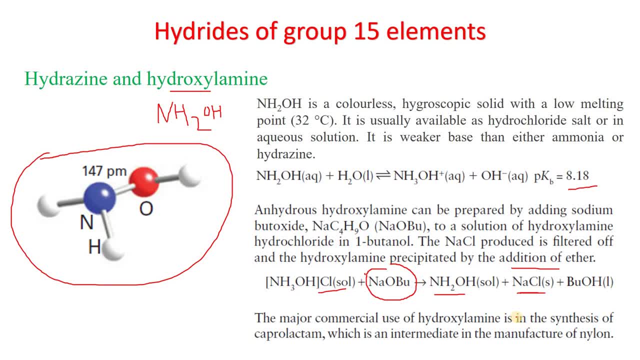 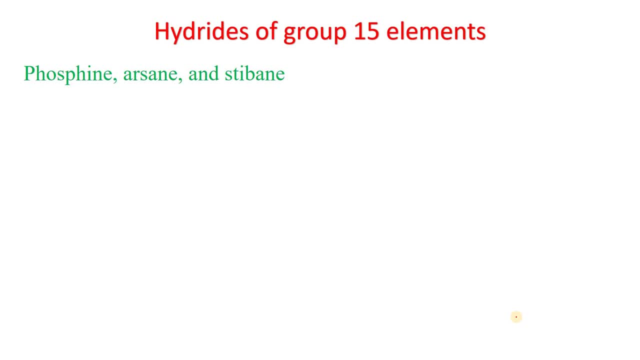 that is, diethyl ether. the major commercial use of the hydroxyl amine is in the synthesis of the hydrides of the other member of the group 15 as a phosphorus, arsenic and antimony. the molecule corresponding hydride are phosphine. 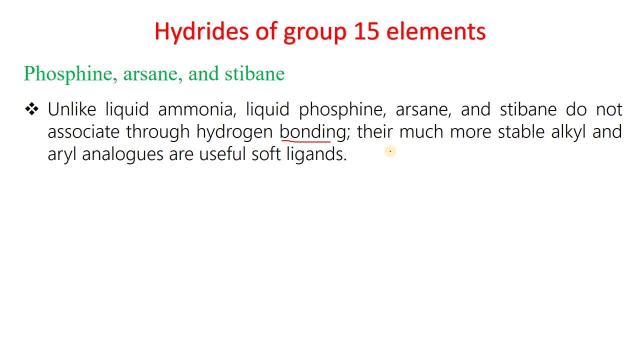 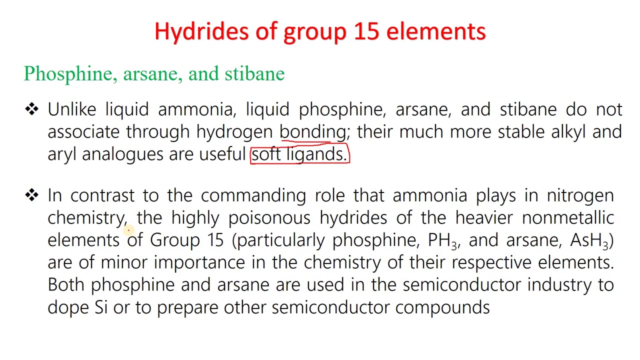 arsine and stebane. unlike liquid ammonia, liquid phosphine are soft ligands. soft ligands are those ligands which have the donor atom, like phosphorus, sulfur and arsenic, in contrast to the commanding role that ammonia plays in nitrogen production of the respective